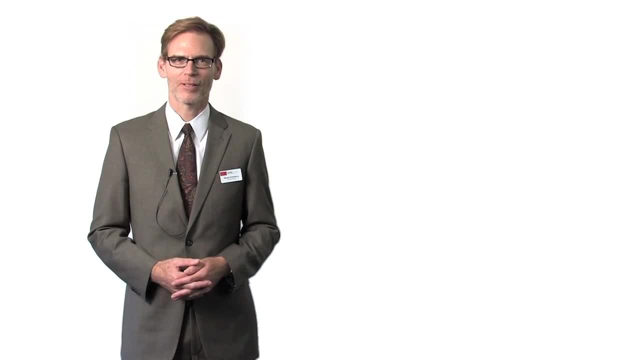 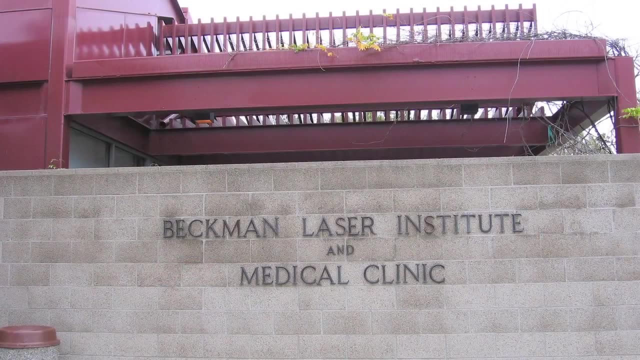 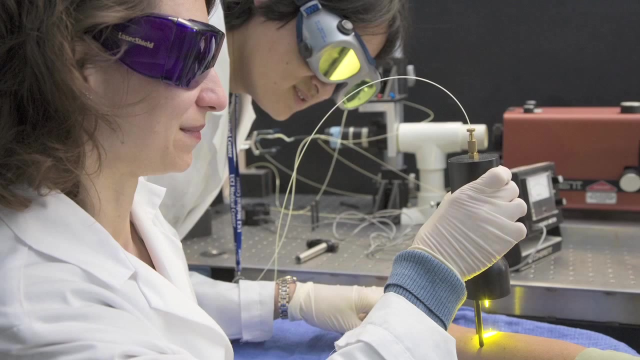 Hi, my name is Bruce Tromberg. I'm the director of the Beckman Laser Institute and Medical Clinic at the University of California, Irvine. We develop a number of biophotonic and biomedical optics technologies. We have a clinic that has 3,000 to 4,000 patient visits per year. 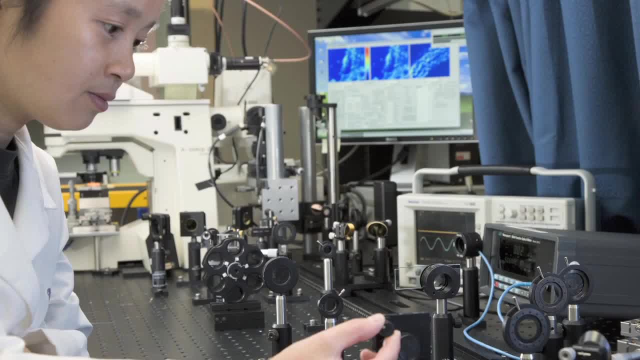 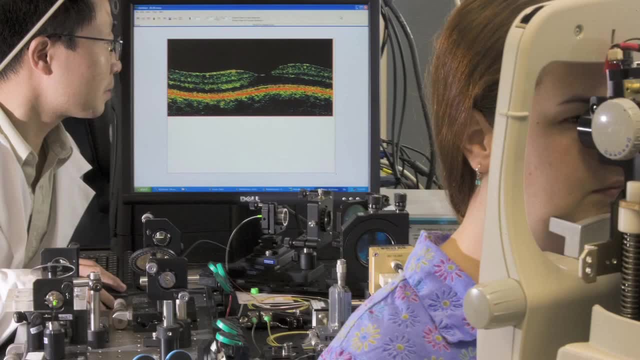 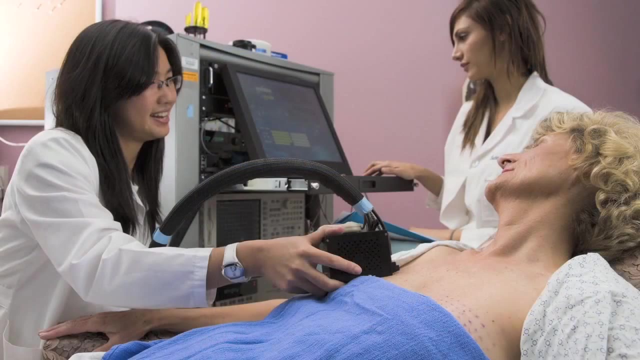 What's very unique about our clinic is that we have a number of IRB Institutional Review Board protocols in new technologies in biomedical optics brought to the bedside. So we're a very unusual place in that we have basic science and technology development labs that are moving. 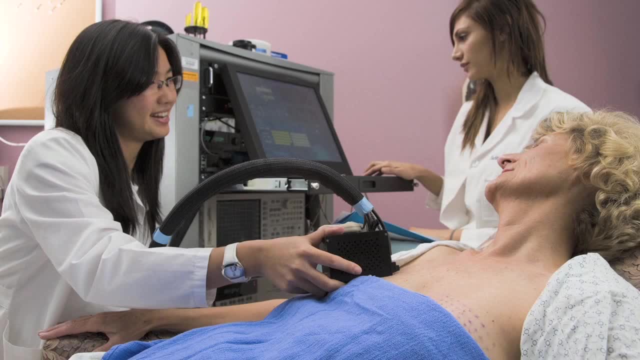 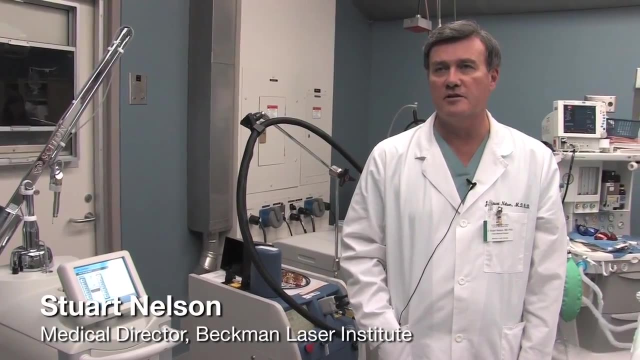 technologies very quickly from the bench top to the bedside. I'd like to take you through the building and show you these. Hi, I'm Stuart Nelson. I'm a professor of surgery, biomedical engineering and dermatology at the University of California, Irvine. I'm also the medical director of the Beckman Laser. 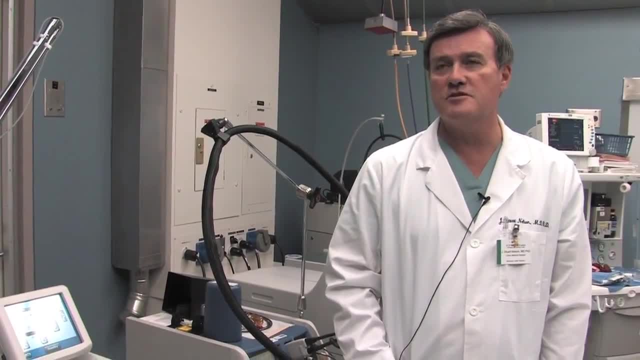 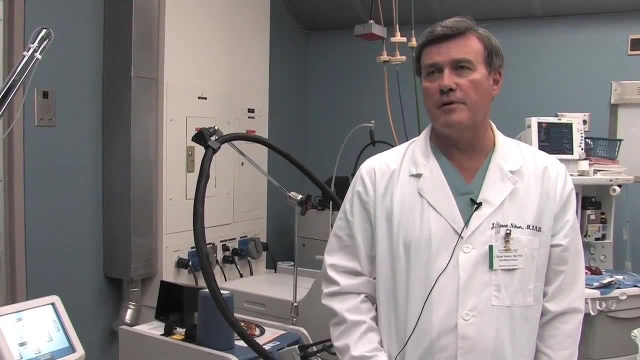 Institute And medical clinic here at UCI. The Beckman Laser Institute was established in June of 1986 by Michael Burns and Arnold Beckman. It was their desire to develop a resource that would be developed and dedicated to the development of laser devices as well as other. 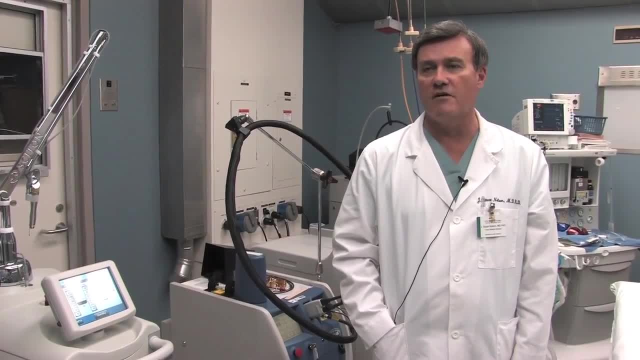 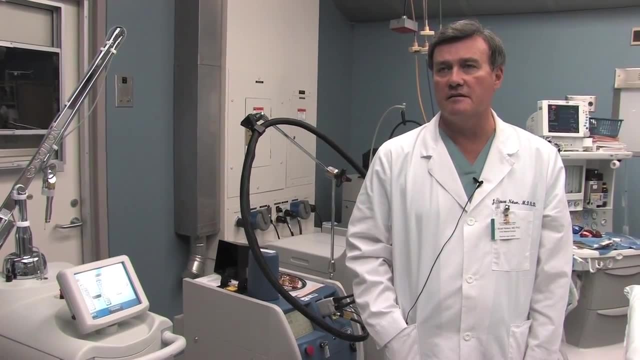 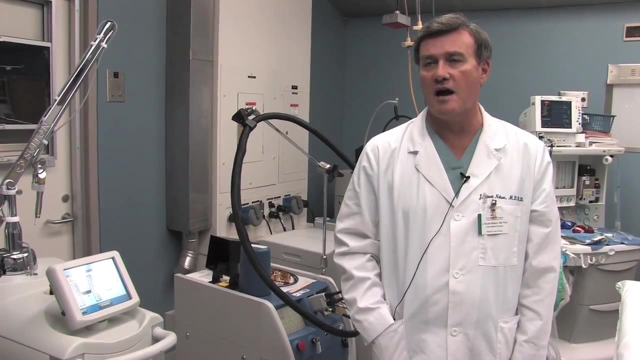 biomedical optical technologies. My research is involved in the treatment of port wine stain birthmarks in infants and young children. These are vascular malformations of the skin that patients are born with. These lesions are progressive. They become darker insidiously over the course of time. 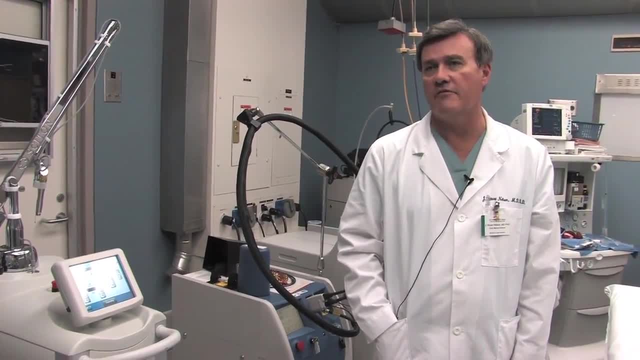 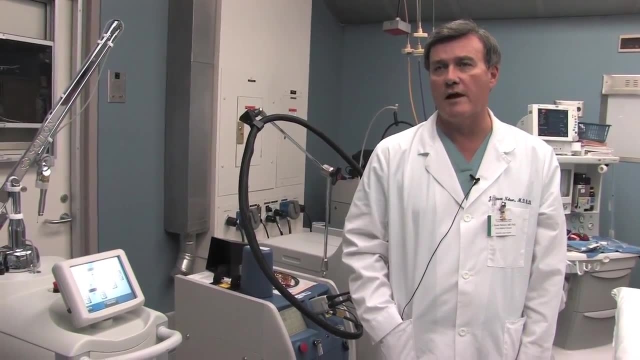 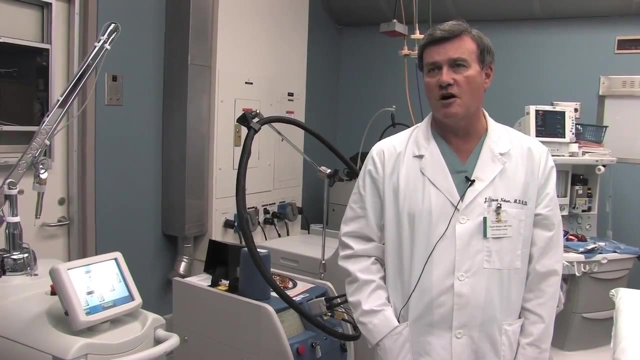 And if left untreated, the patient can develop soft tissue hypertrophy of the underlying soft tissue, muscle and bone, which further distorts their facial features. So the goal of my research program has been to develop novel and new technologies so that we can treat these birthmarks more effectively, while treating patients also younger, so that they 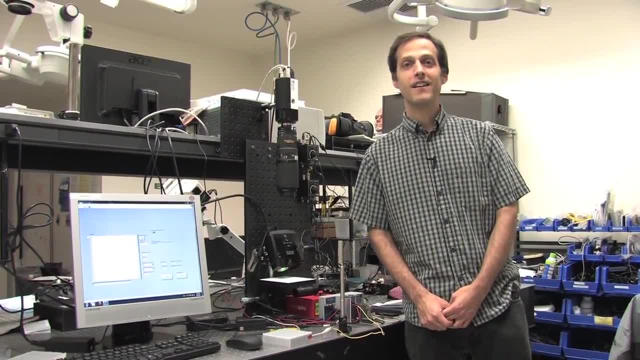 can get the most benefit from the treatment. Hi, my name is Soren Konecki And I'm a postdoc here at the Beckman Laser Institute. I'm a postdoc here at the Beckman Laser Institute And I'm a postdoc here at the Beckman Laser. 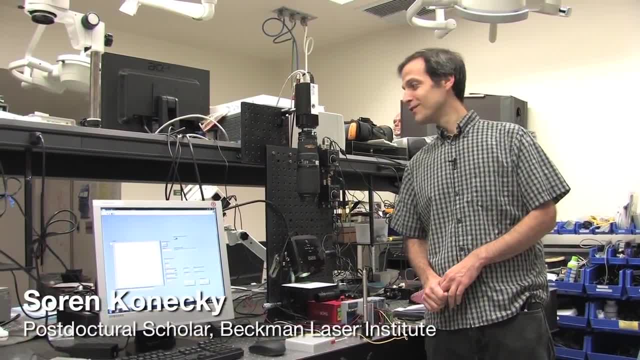 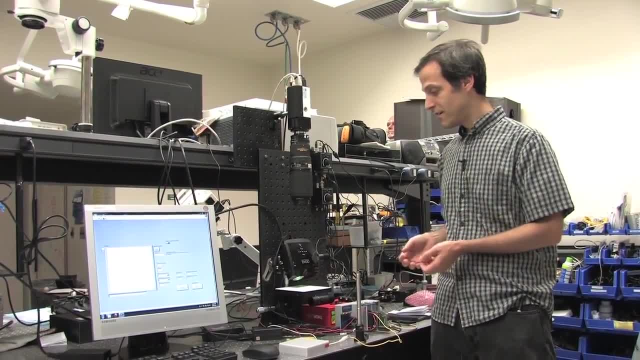 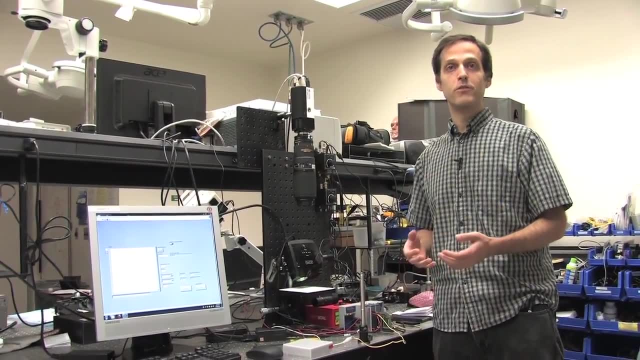 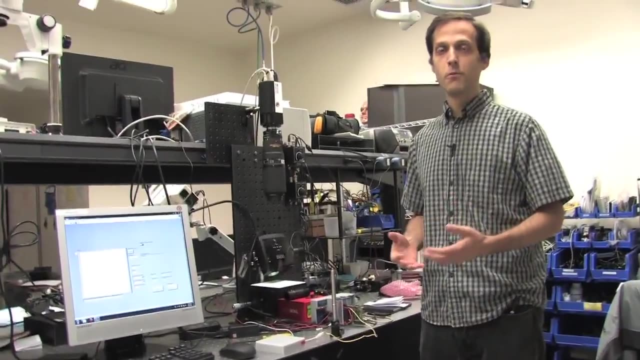 idea is: we have a camera here and we want to combine the benefits of photography- that is ubiquitous in both medicine and biology- with the benefits of diffuse optics, which is a spectroscopic method to get precise measurements of the concentration of chromophores in tissue. 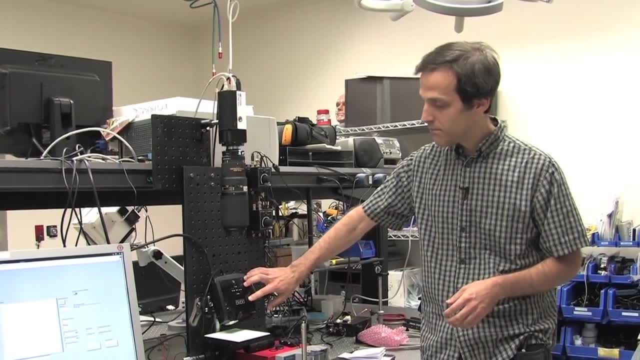 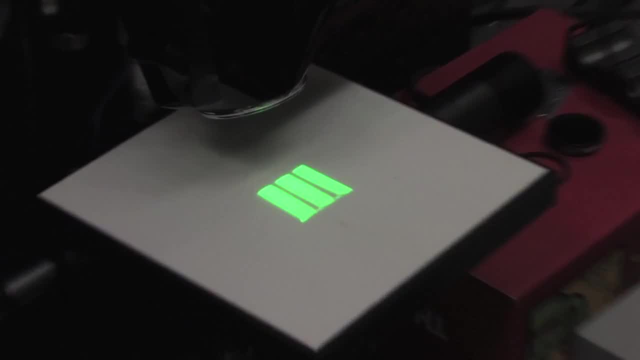 and the optical properties of the tissue. If you see, here there's a projector That basically is projecting sine waves of intensity onto a sample And by measuring how those sine waves blur as they go into the camera, then we can get the tissue optical properties. 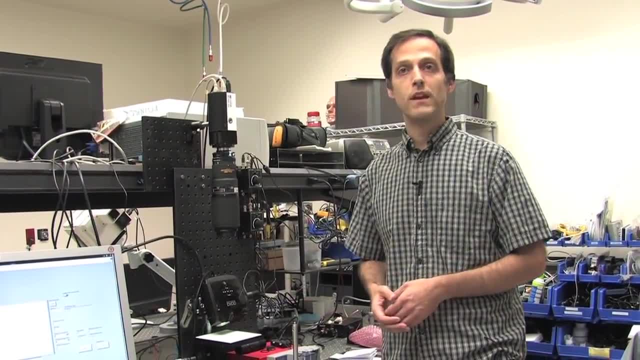 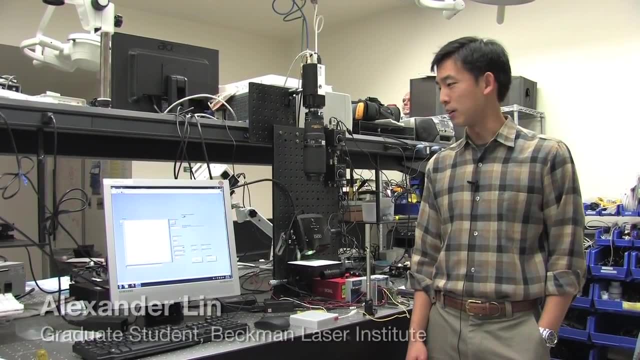 But the great thing about it is then we get a photograph too, So we get a quantitative photograph of the tissue. My name is Xander Lin and I'm an MD-PhD student in Bruce's lab, And my project is to image. 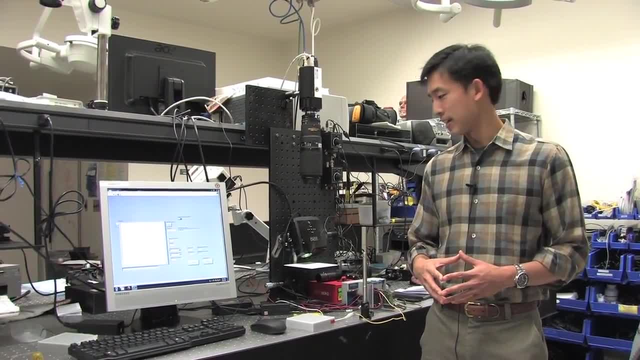 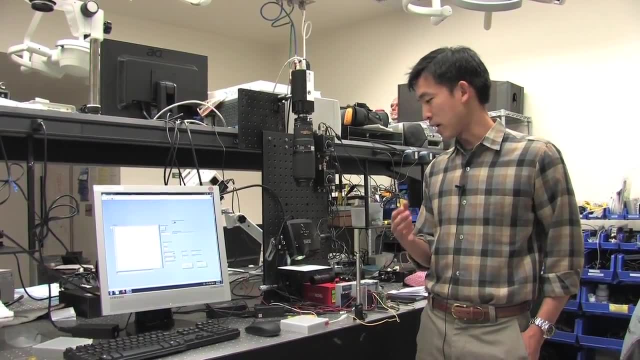 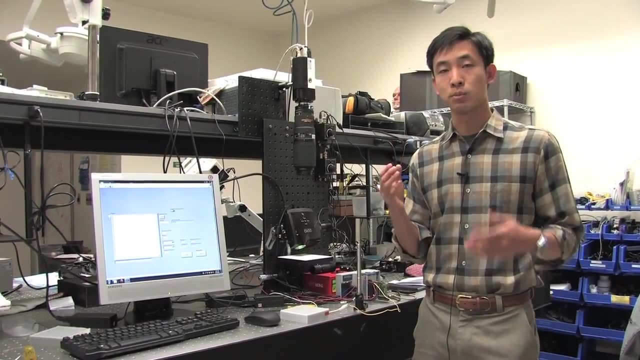 Alzheimer's disease in a preclinical model. It's a mouse model, And so we look at the hemoglobin, oxydeoxyhemoglobin, and how it functionally changes when we stimulate certain parts of the brain, And we hope to see differences. 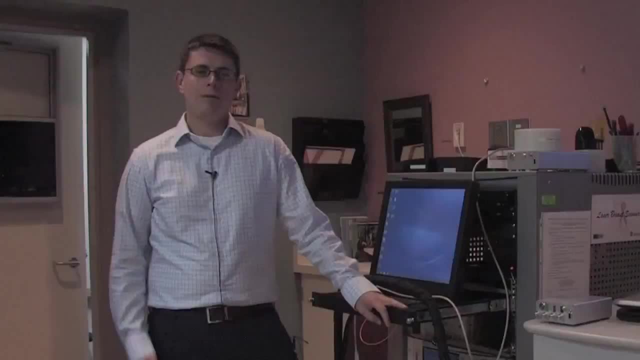 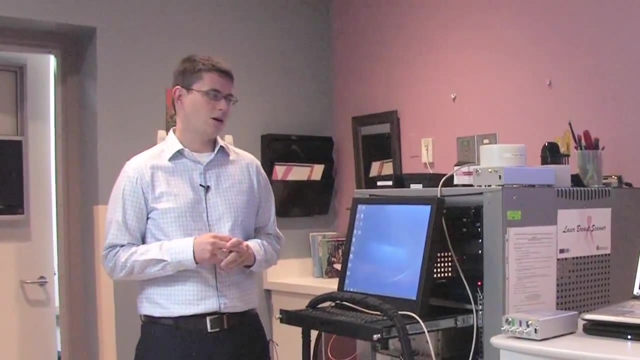 between a regular mouse and an Alzheimer's mouse. My name is Darren Robilaire, I'm a postdoc at the Beckman Laser Institute, working for Dr Bruce Traumberg, And today I'm going to be showing you a little bit about our DOSI. 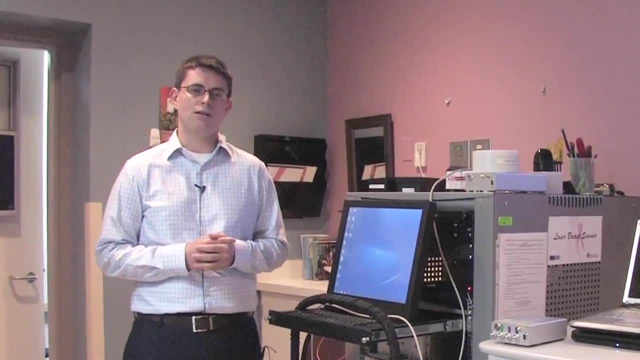 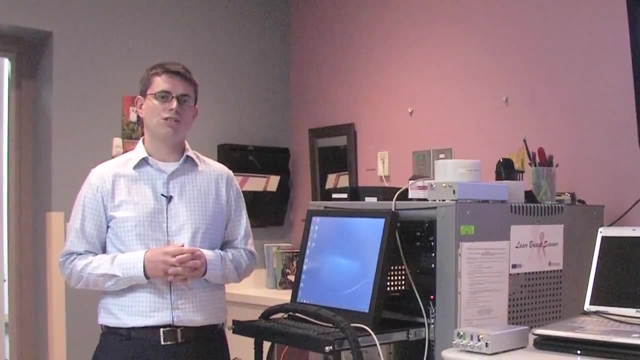 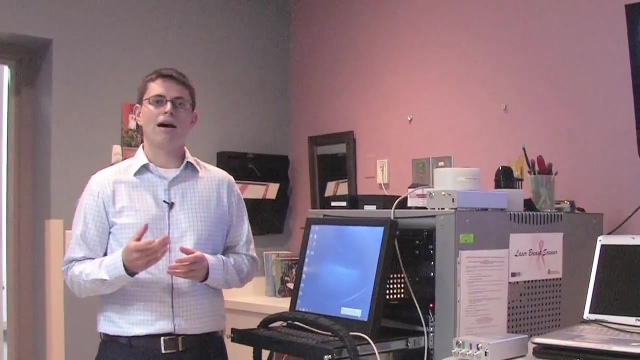 technology That stands for Diffuse Optical Spectroscopy. This is an instrumentation that allows us to inject a tumor into the brain through microscopic imaging, And this instrumentation we use to get functional properties from thick tissues such as breast tissue, So we can extract properties such as oxydeoxyhemoglobin, water and fat. 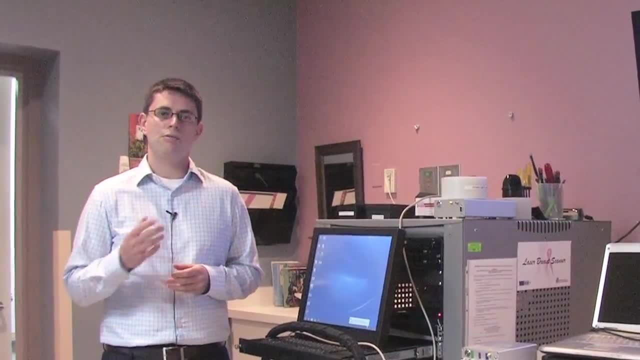 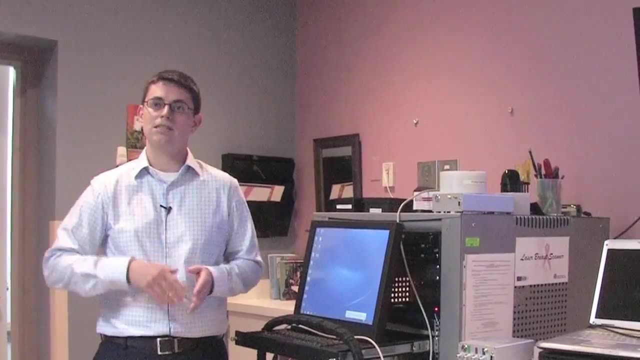 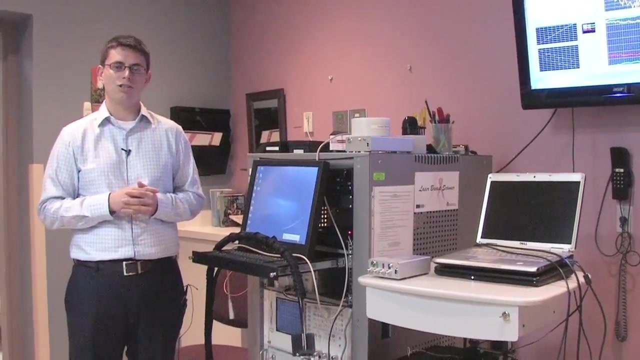 And we use this technology to monitor patients, specifically breast cancer patients, while they're receiving chemotherapy, typically before their surgery. So we use this technology to monitor those functional changes during the course of therapy. to see and predict is based, in addition to lasers, on RF technology, and this is our last generation device and 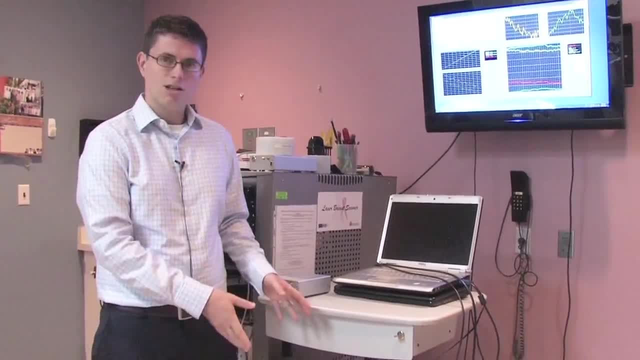 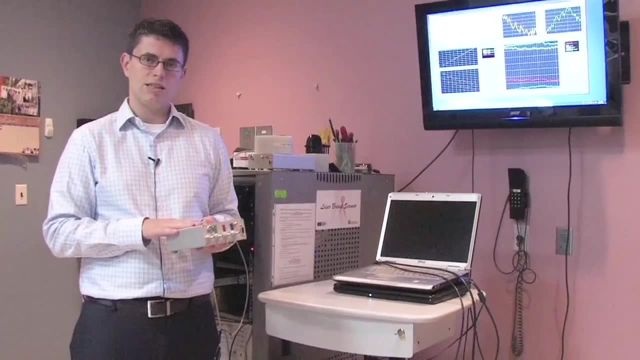 we've been able to miniaturize this instrumentation so that it's the size of a microwave now, or even the size of about an external hard drive. So the capability in this box is approximately equal to the capability of this large device. My name is Thomas Sullivan. I'm also a postdoc. 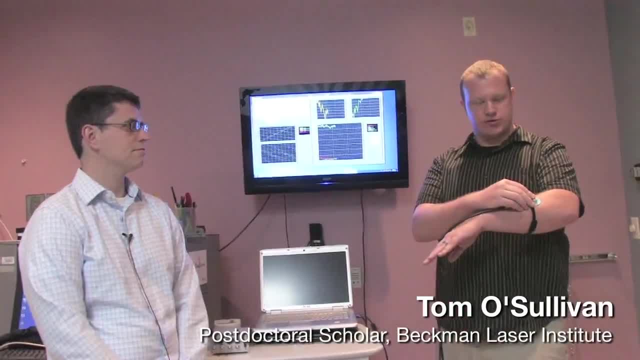 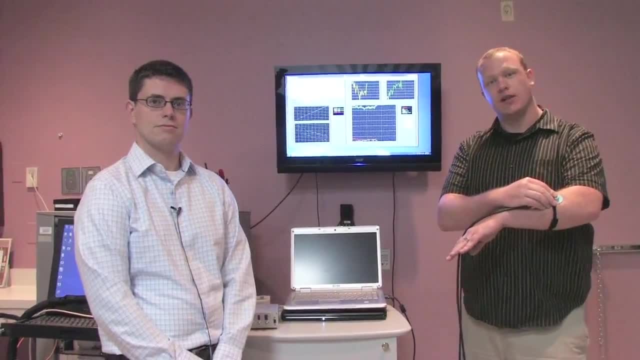 here at the Beckman Laser Institute. I work for Dr Bruce Tromberg along with Darren here, and together we're going to demonstrate our real-time functional spectroscopic imaging technology dosing. So using this new technology, we can, as I mentioned before, get quantitative. 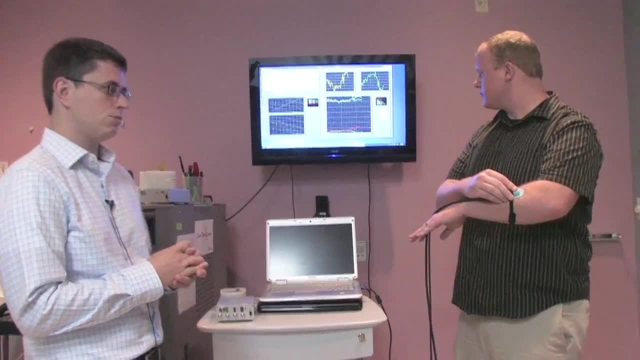 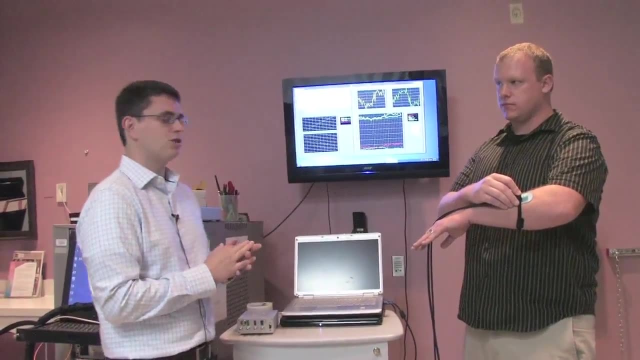 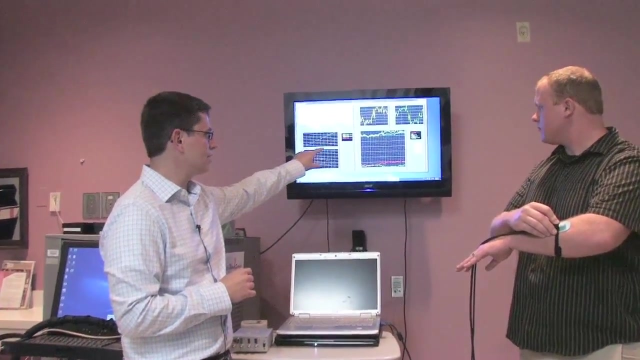 values of oxygen deoxyhemoglobin, water and fat from tissue. So Tom has a probe on his arm that's measuring photons that are penetrating through his muscle and on the screen here we're displaying real-time images or real-time data of oxygen deoxyhemoglobin. 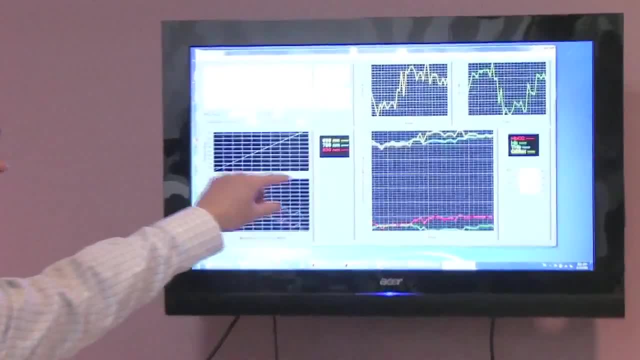 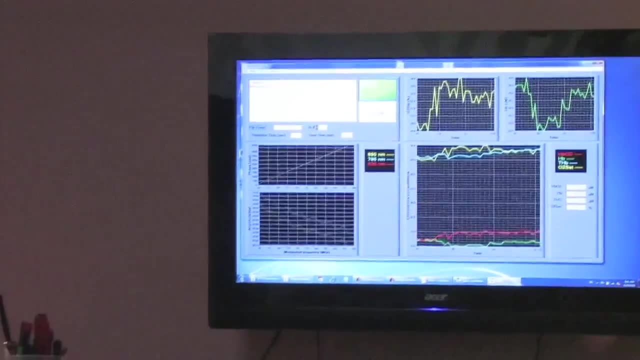 Oxi is in the red and deoxy is in the green, as well as oxygen saturation and total hemoglobin, And we can look at that over time and we can do this in, say, diabetic patients to determine if their utilization of oxygen is equivalent to, say, a normal volunteer, to. 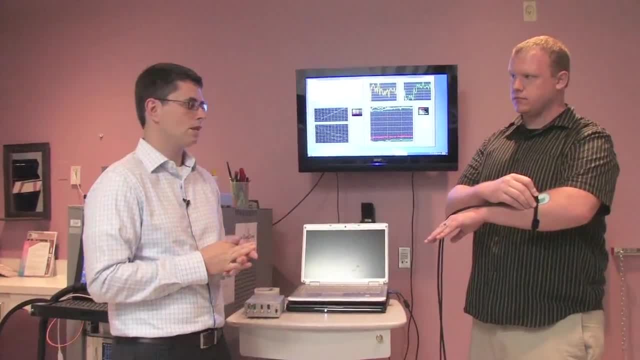 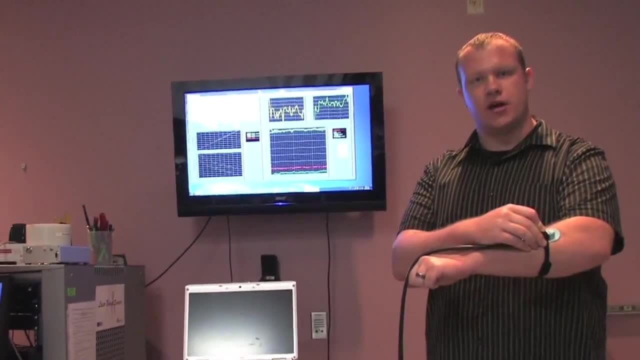 help develop diagnostic methods or to help understand biology better. This is based on the same technology we use in our breast cancer patients and, in fact, this exact system we take up to the chemotherapy infusion center regularly. because we're using the same technology we use in our breast cancer patients and, in fact, this exact system we 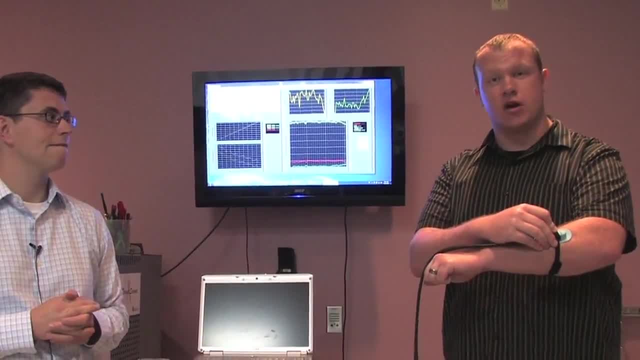 use in our breast cancer patients and, in fact, this exact technology we use in our breast cancer patients and, in fact, this exact system we use in our breast cancer patients, because we want to study, on a very short time scale, the effect that these drugs are having on these patients, with the goal of being 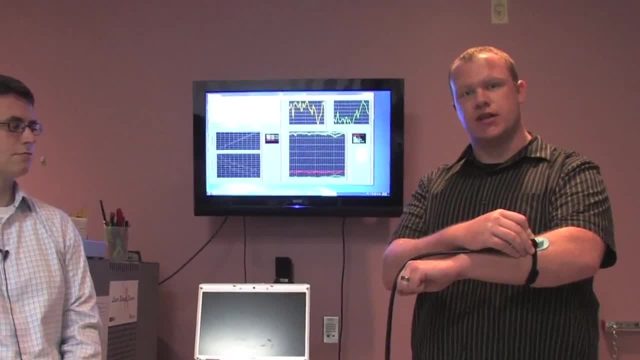 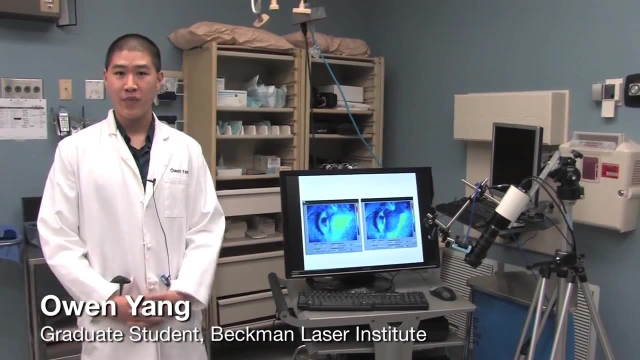 able to very early predict the efficacy of those drugs in that setting. Hi, my name's Owen Yang. I'm a graduate student here at Beckman Laser Institute and I work in the Laser-Speckle Laboratory, And the project that we are working on right now is using 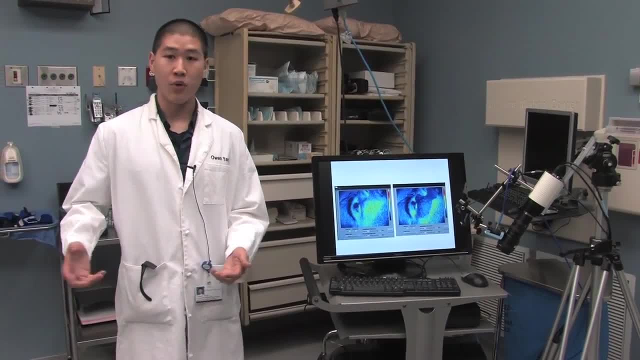 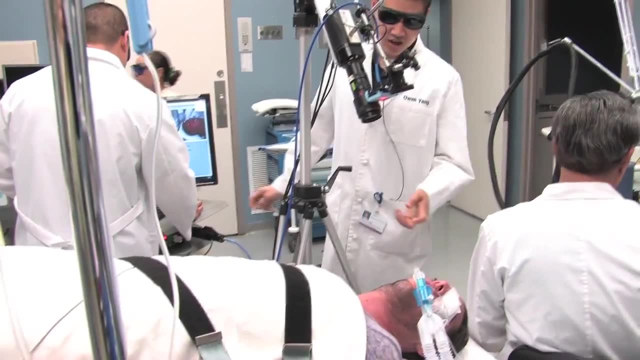 Laser-Speckle as an instrument to help treat pole-weinstein, to give an indication on whether or not blood vessels have been coagulated successfully post-treatment. So just to talk a little bit about the system. it's a laser speckle system. We shine a laser on 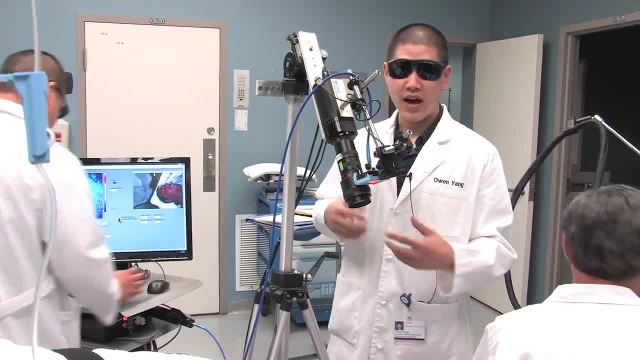 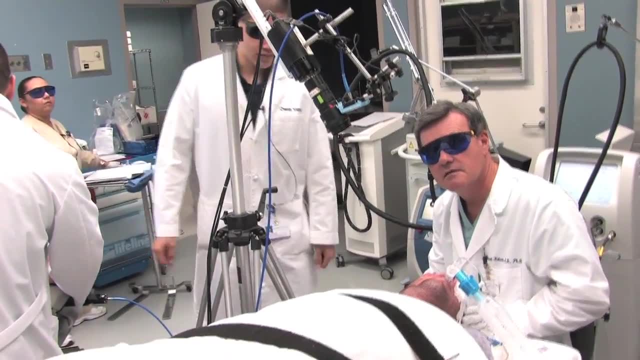 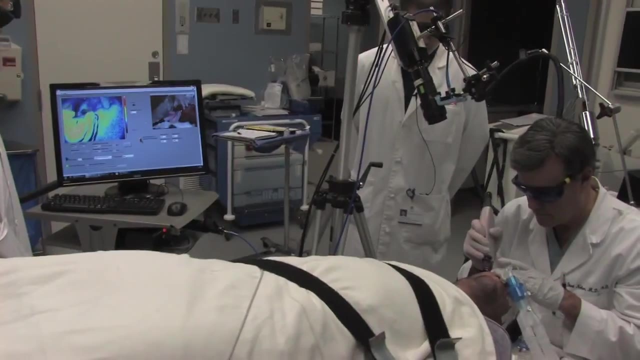 the surface and the light that comes back will give us information about how much blood flow there is on the surface of the skin, where mostly the blood perfusion. This is a port wine stain patient, so I'm going to use the pulse dye laser to coagulate the blood vessels underneath the skin and the skin will look bruised as a. 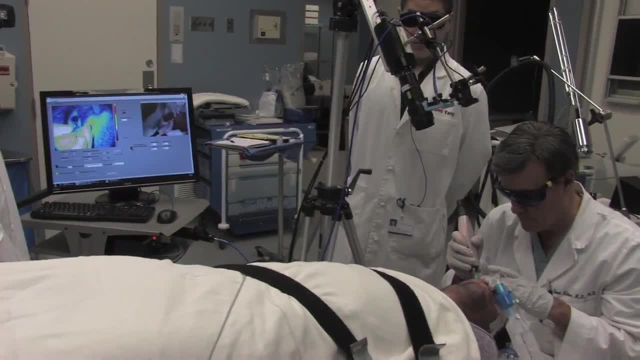 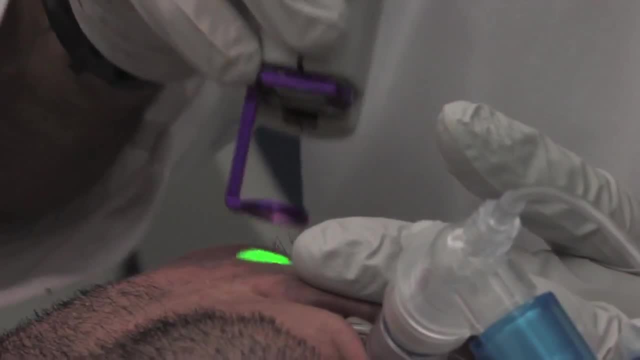 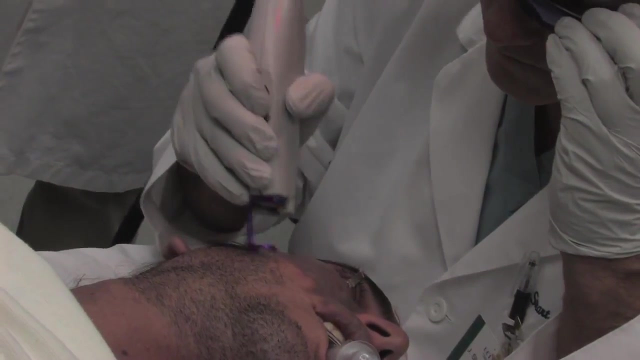 result of me doing the laser treatment, But what we're looking for in the images is the reduction in blood flow that will tell me that we've clotted the blood vessels successfully underneath the skin. So hopefully, after the treatment, you could see coagulation of the blood vessels and a decrease in flow, which we should be able to see on this using this laser speckle system. 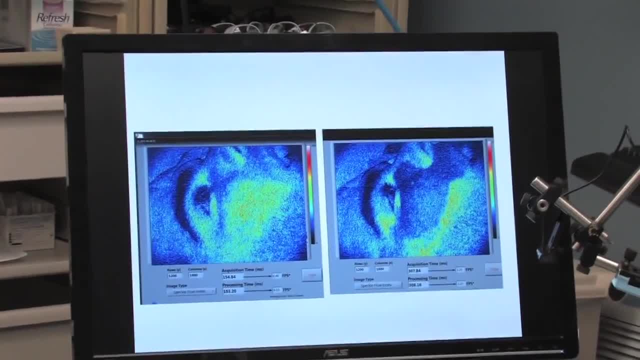 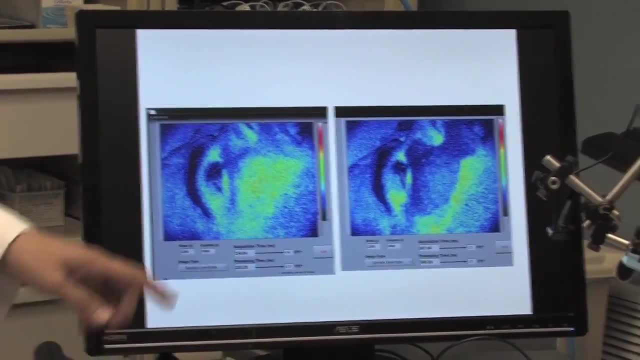 And you can see these brighter colors indicating more blood flow, which is what you expect in a port wine stain, because you have dilated blood vessels. you have more concentrated blood vessels in the area of a port wine stain, which is seen here with the brighter color. 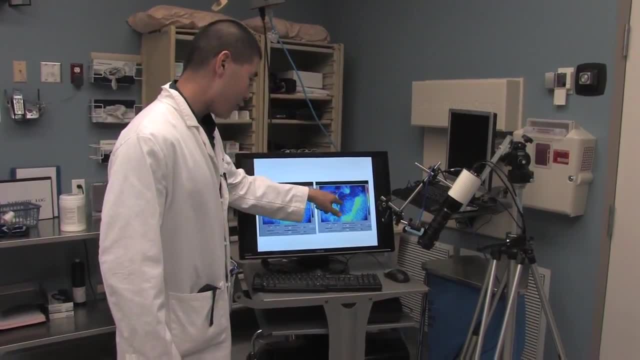 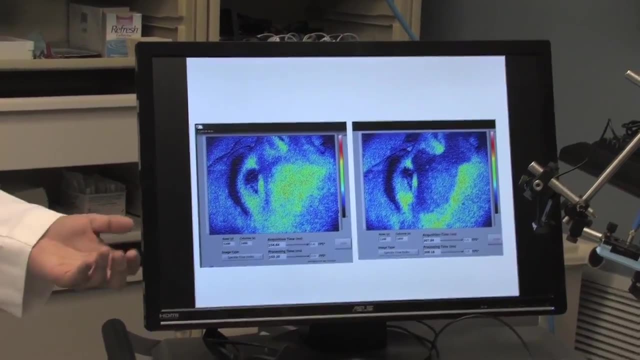 What you want to see is this image here on the right where you have, after treatment, a darker color in the area of treatment, where that indicates you have less blood flow, which is exactly what we want. And if, if you were to see areas of brighter colors, that would probably indicate that you did not successfully. 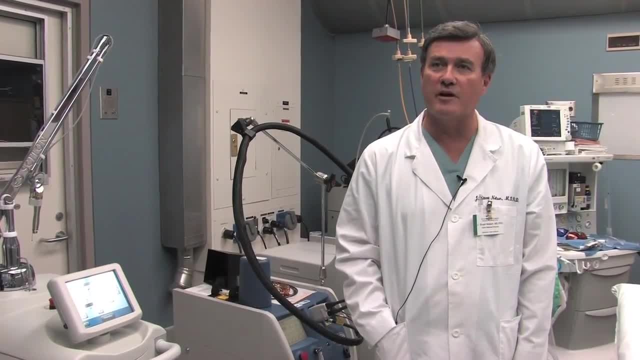 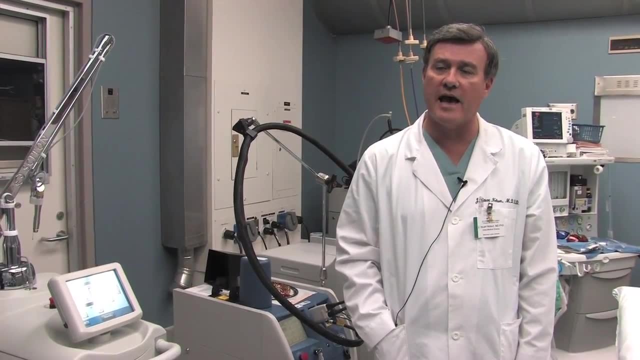 coagulate those regions, As our director, Bruce Tromberg, likes to say, from benchtop to bedside, because we literally can take technology that our basic scientists develop in the labs and then bring it down the hall on this side of the building where it's applied in the clinical management of patients. 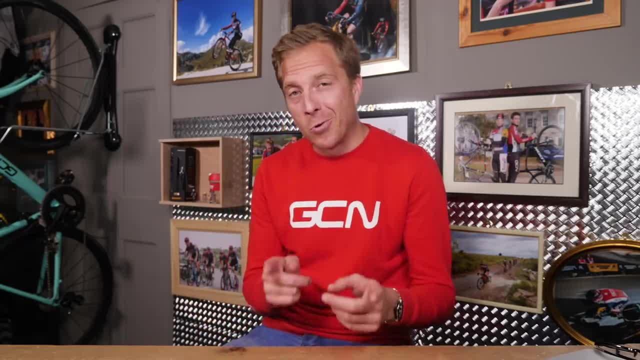 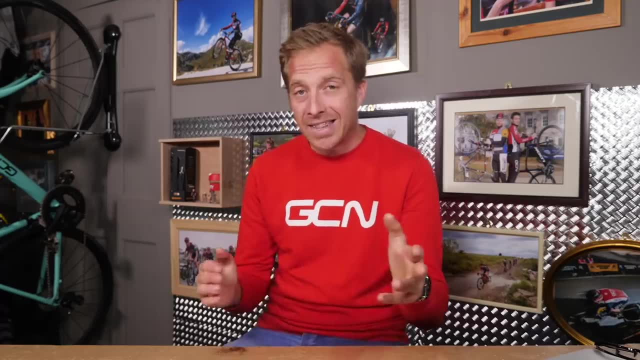 Now, you may not be aware of it, but you could well be destroying your bike, Sometimes in an instant, and sometimes just accelerating the natural wear of components. Today, then, we're gonna look at some of the ways in which you could well be destroying your bike. 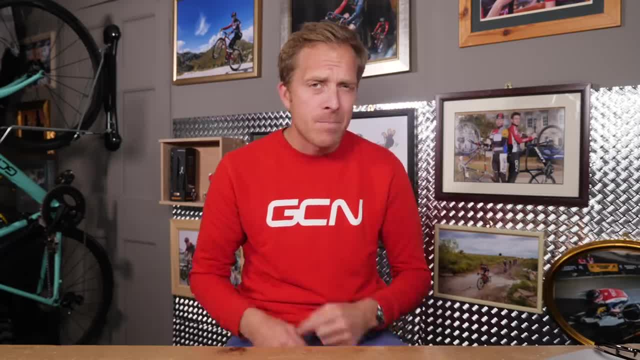 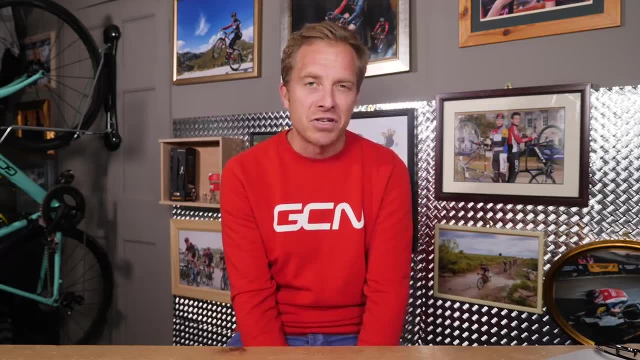 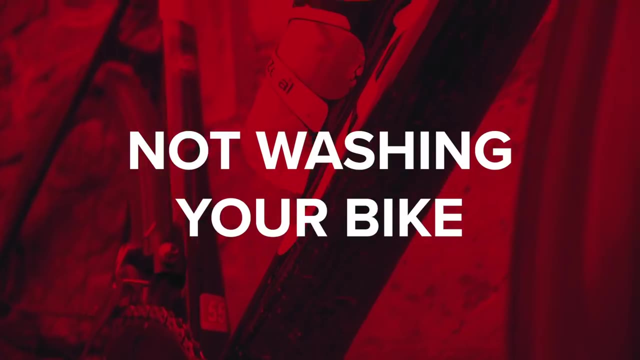 and, importantly, how to combat it. But before we go on, make sure you subscribe to the GCN Tech channel and also click that little notification icon and bell so you get alerted each and every time we put a video live- Now, not every time you wash your bike. 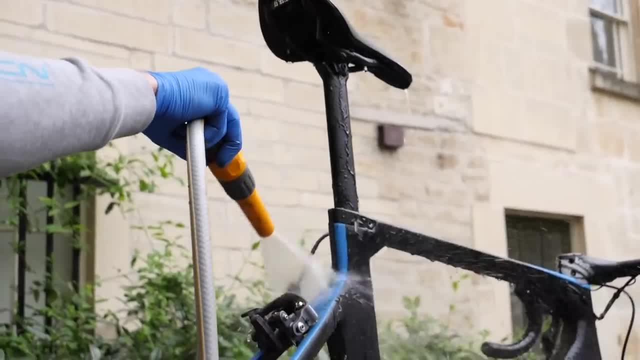 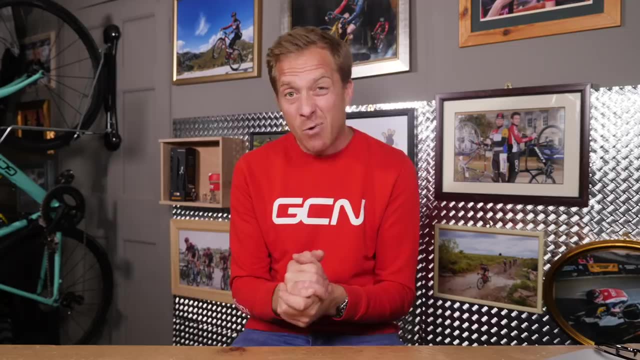 does it have to be a very thorough affair, but I would recommend certainly every couple of months to give it a very good going over. Try and get it to look as new and as clean as possible. That way you're gonna uncover any potential disasters. 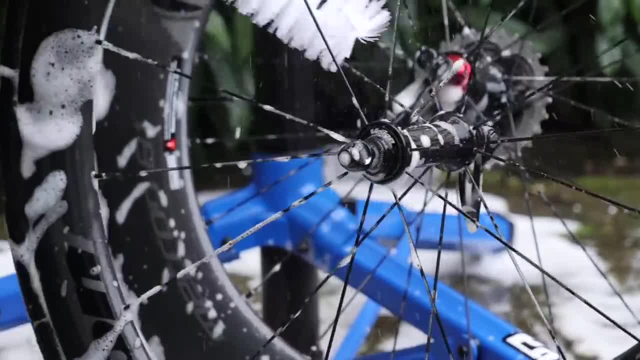 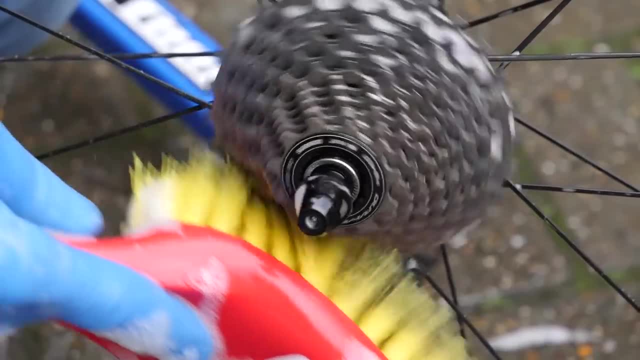 that have been hiding underneath the dirt and grime. Plus, you're less likely to have any mechanical faults going on, because it's gonna be working smoothly. And, besides, a clean bike is a fast bike and a clean bike is a bike. 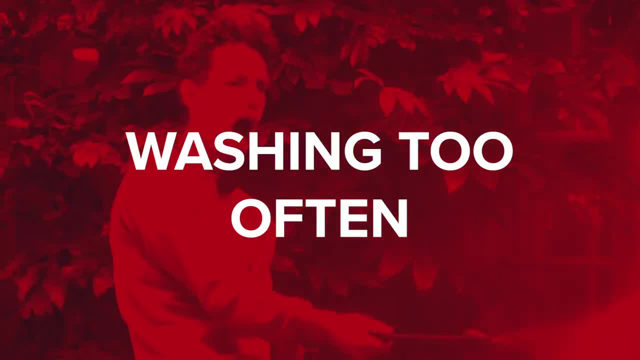 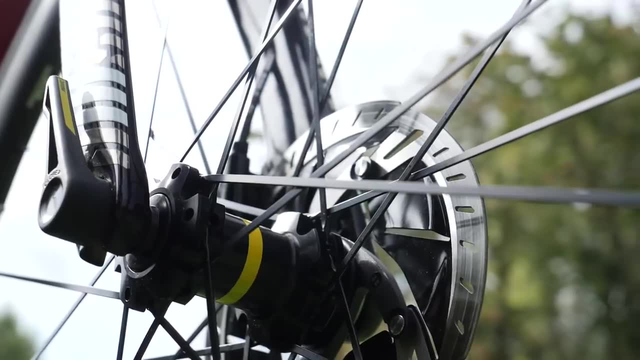 that you're gonna wanna go out and ride on. That's right. if you go ahead and wash your bike after every single ride, trying to get it to look like it should be inside of a catalog or something, you could well be doing it more damage than good. 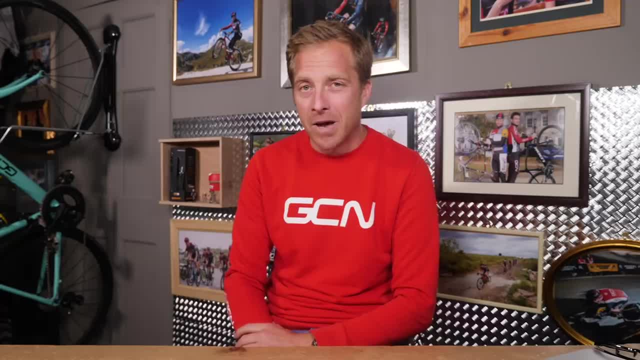 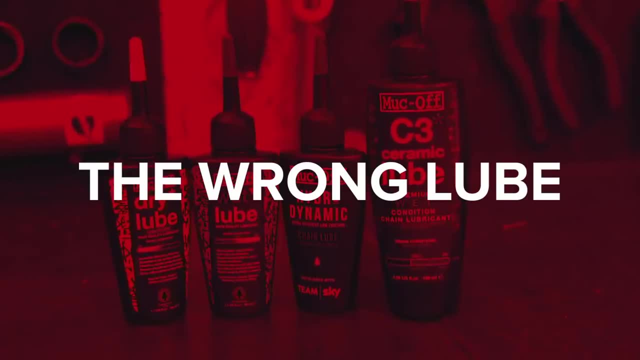 you could be removing all of that useful goodness inside of the components and, well, replacing it with nothing. Best leave it to when it actually needs doing. Many times people head out on a bike ride and they look down at their chain and think: